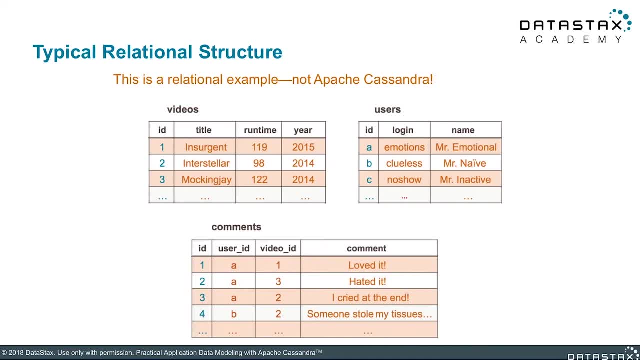 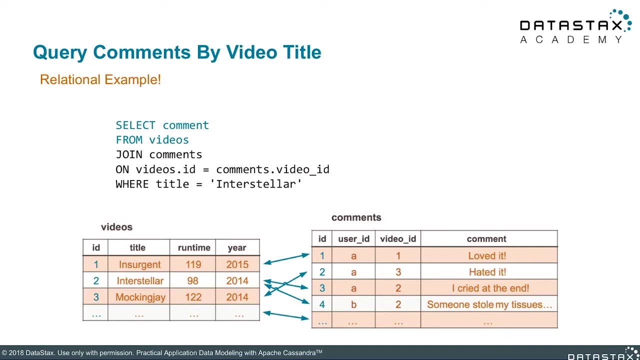 to do a query to join those together. How does that work? In this case, I want to find some comments for a particular movie. If you look at those two tables, you have comments in one, you have videos in the other, so that data exists in two different places. So whenever 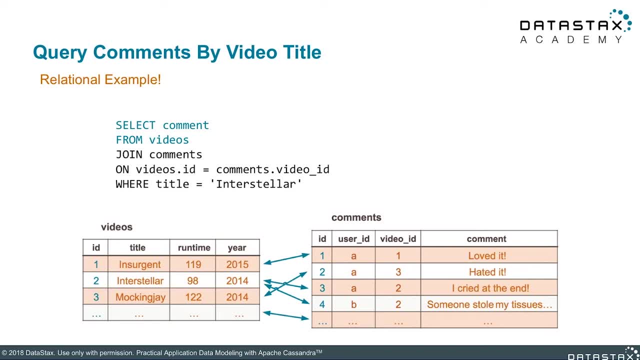 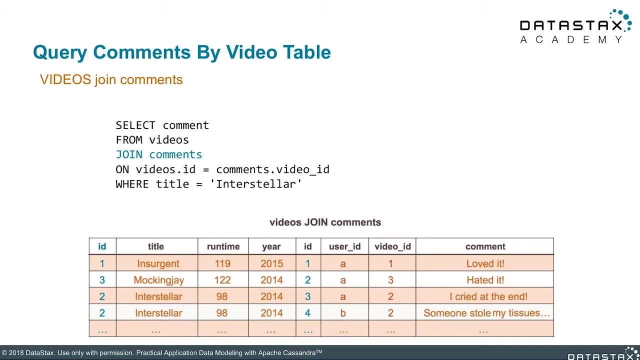 I select a comment from videos. how am I going to get that comment out if I just had the video? So I'm going to use the join statement. That join on comments is going to join those things together. The join statement. Now, that is how relational databases work In. 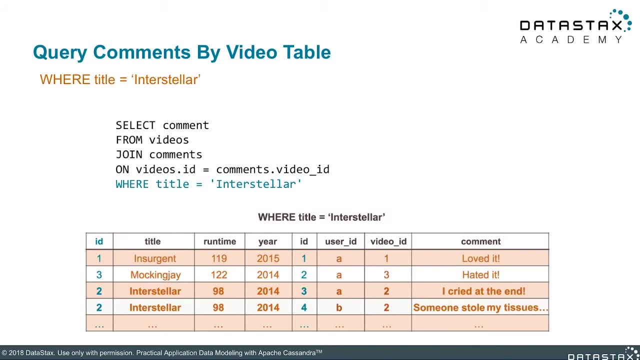 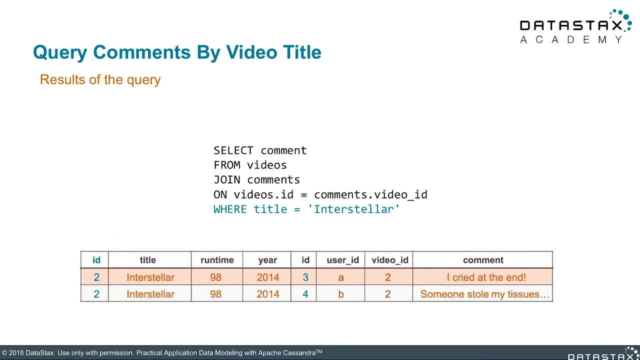 this case I say the title is equal to interstellar. I know that I can use that to do a join on those two tables and get the comments just for that one title. That is how relational databases were designed, having multiple tables And then in the query, that's when I start. 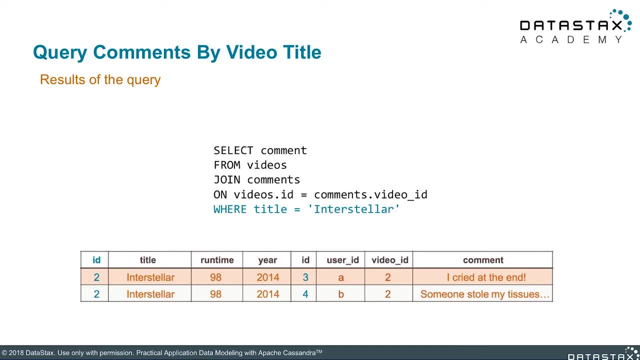 building these things together. So the results of this query In this case will be: if I want the title of interstellar, I get the comments just for that one movie, but the join happens in the database. What about something a little more? 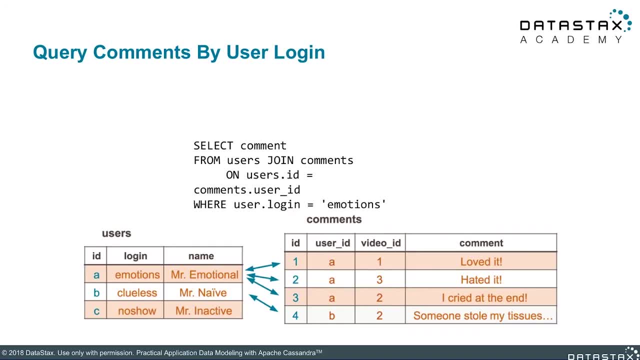 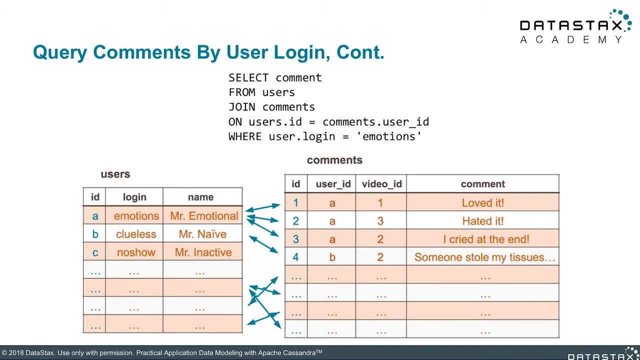 complicated, Maybe something like logins. We're looking for particular comments by a user. So here's this: user emotions, and we want to find out every comment that that user had put into the system. Again, another join, So in this case it's just a few, but what? 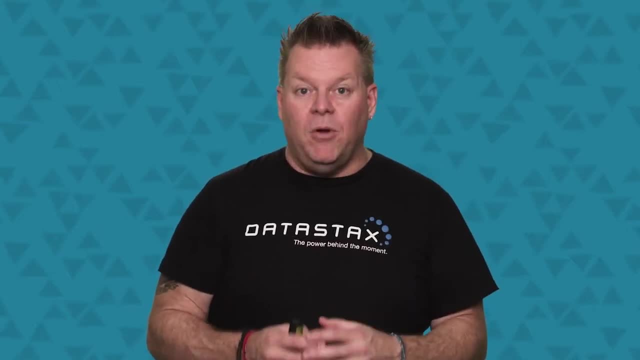 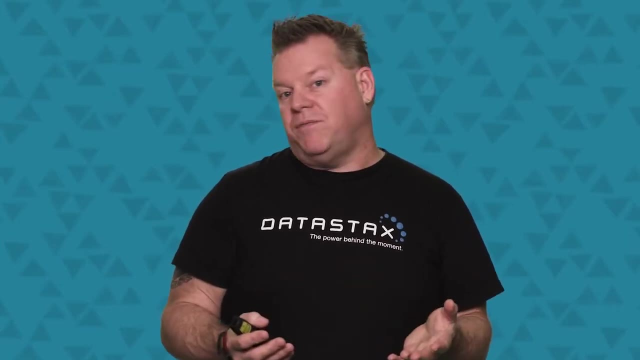 if it's a lot more. Well, there's the problem with relational database modeling is that eventually you're going to run into the situation if you're not careful- And, let's face it, you don't know when it's going to happen- but eventually you're going to see that there's too many. 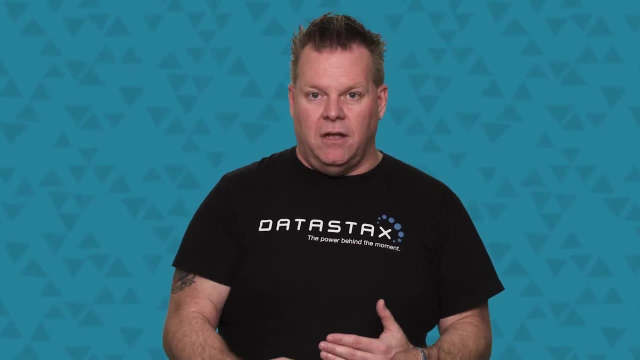 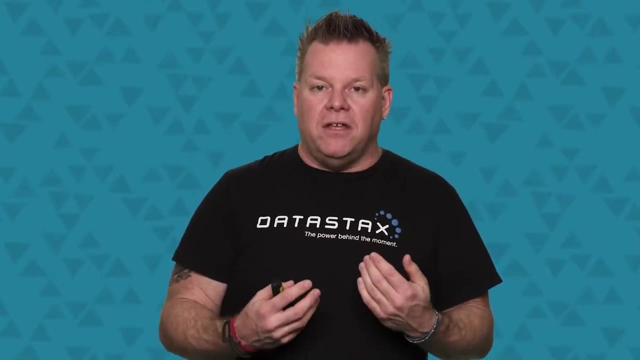 records in the join and it'll start slowing down your queries A lot. I've run relational databases for years and years and this is the thing that we always try to avoid, And of course, you do things like add indexes to it or maybe truncate some data, which 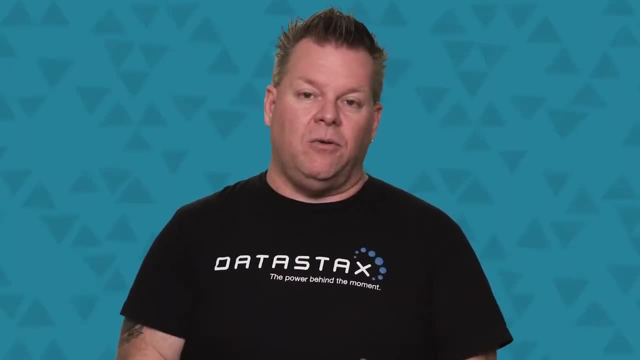 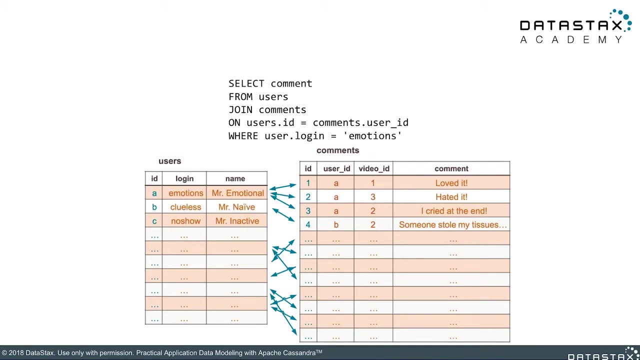 is really bad. You could do that. Or another thing that we did quite a bit with relational databases, That is denormalizing. Denormalizing is a really common technique, even with relational databases, but it's a really critical task with Cassandra. If you look at this diagram, you see these two queries. 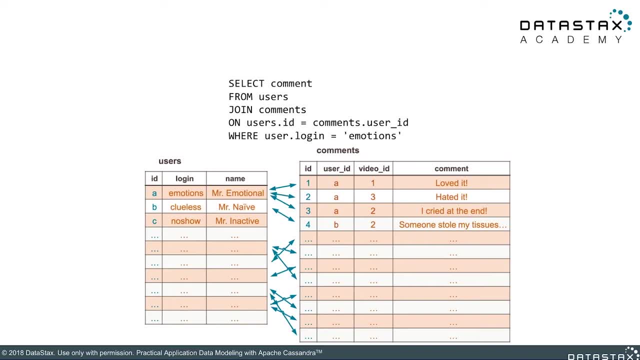 that we needed now represented an entire table, So we want to find all the comments for a video or comments by a particular user. Those are now tables and those tables store all of the data you need And if you look at these tables, they look really similar and there is a duplication. 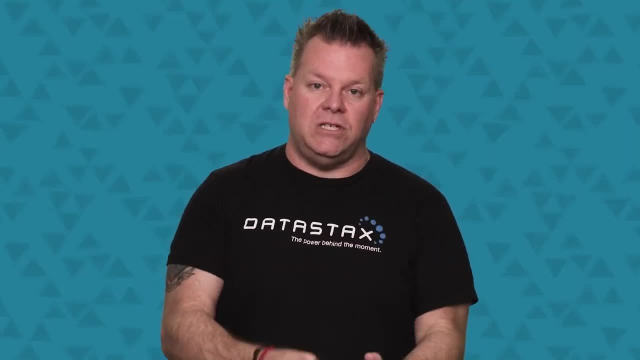 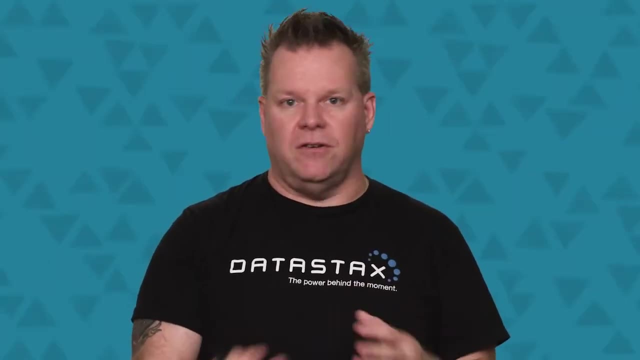 of data. Here's the thing you need to be okay with. When you denormalize, you're going to have duplicate data. That's okay, Because you need data when you need it, not whenever the server is ready to give it to you. Or hang on, let me go do this really complicated. 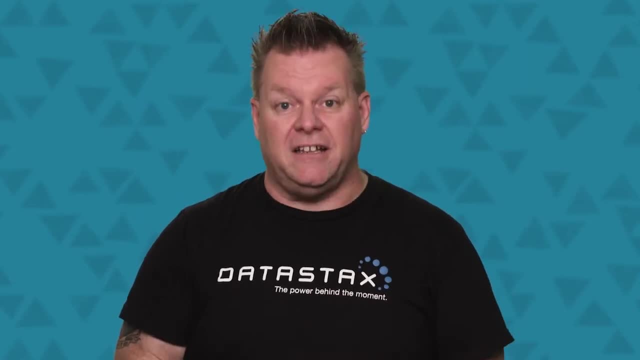 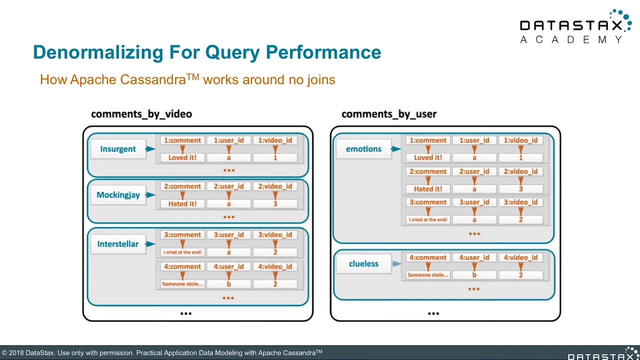 join. Have you run an explain plan? It's probably a little expensive. This case, you know exactly what you're getting. Looking at these two tables: yes, they're very much the same. However, look at the primary key. The primary key is very different Because in the first one video title is the partition. 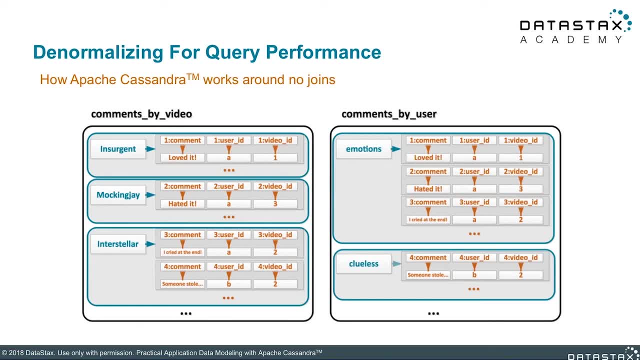 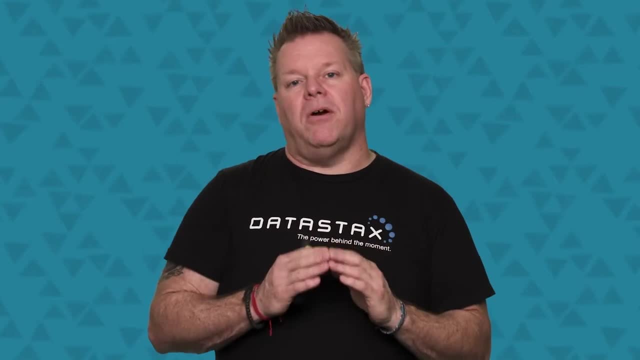 key Comment ID is the clustering column. The other table comments by user. the user login is the partition key. The comment ID is again the clustering column. The subtlety here between those two data models is the partition key. What's that primary part of? 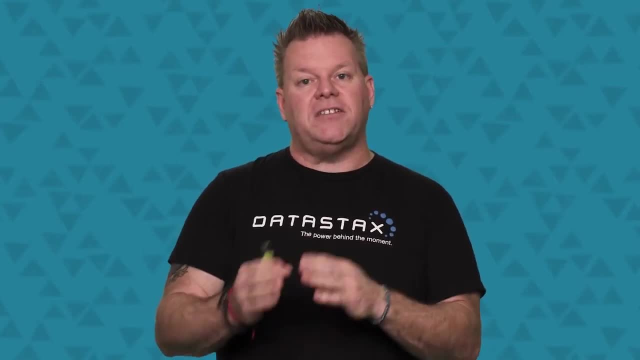 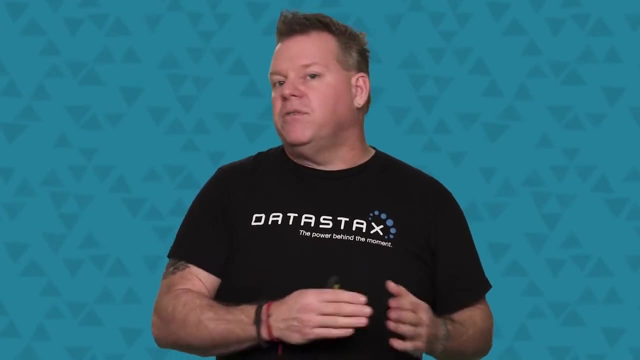 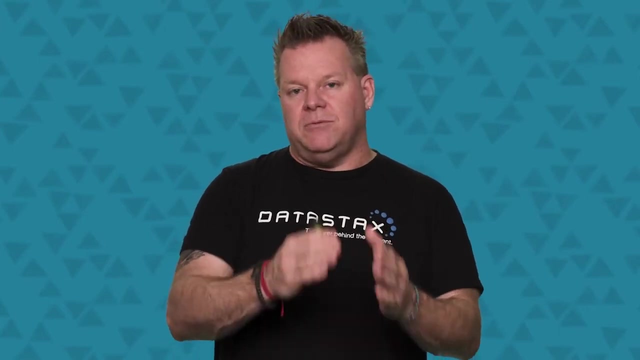 that record It's the person or the video, And then the clustering column gives you the run out of everything that's happened for that video or for that person. That's a really super-efficient data model And it works really well in the Cassandra world. And these are denormalized tables now of that same join. 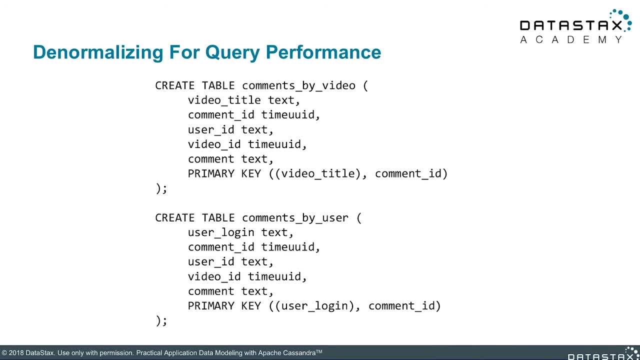 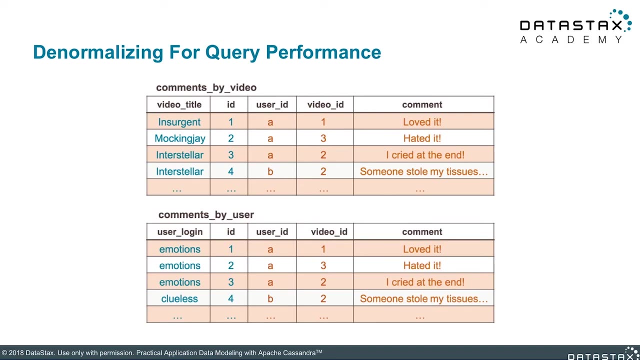 that you had to do in a relational database. What it gives you is this really efficient and predictable query performance. So if I look at the query result for comments by video or comments by user, you get rows and columns in a very sequential way, but it's very fast. 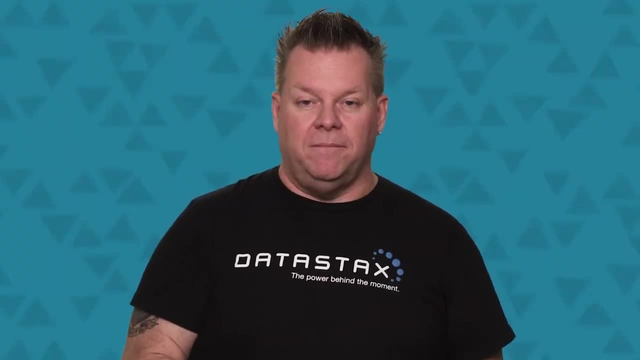 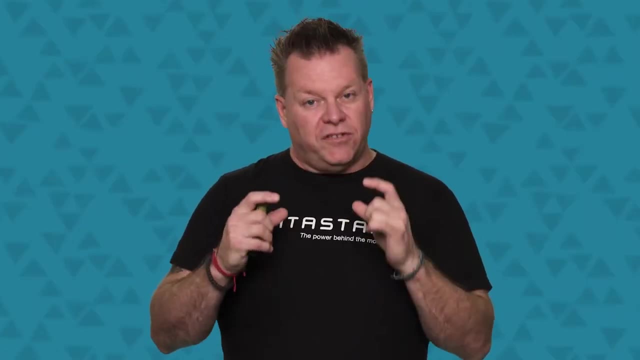 This is the key to high performance with a Cassandra data model- is not only understanding the partition key and how that works by putting your data in the right place, the clustering column with a sort order- what is it going to look like on disk? but then, finally, how? 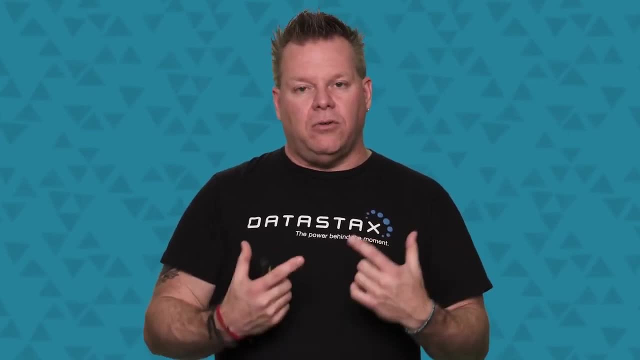 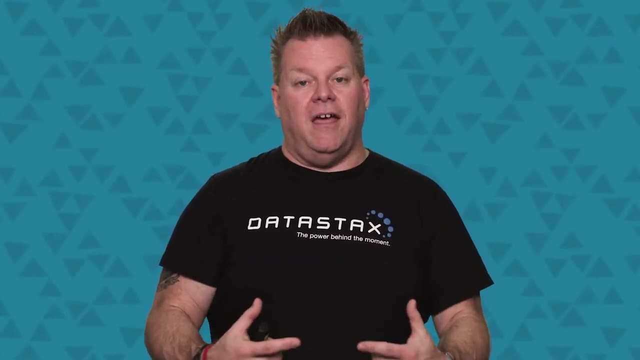 do I denormalize my data? Denormalizing is a really critical part of the plan. You're going to be optimizing for certain queries in the way that you need it, when you need it, And sometimes- I'm going to say this again- you're going to have duplicate data. Then